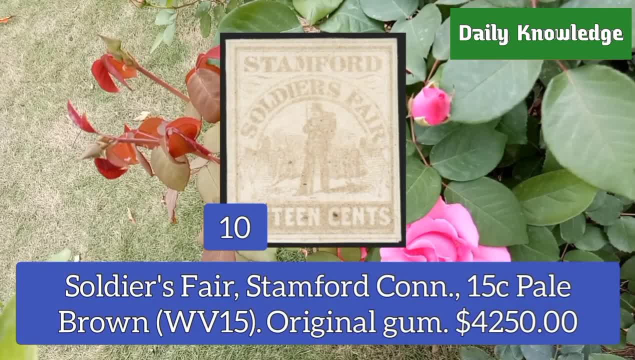 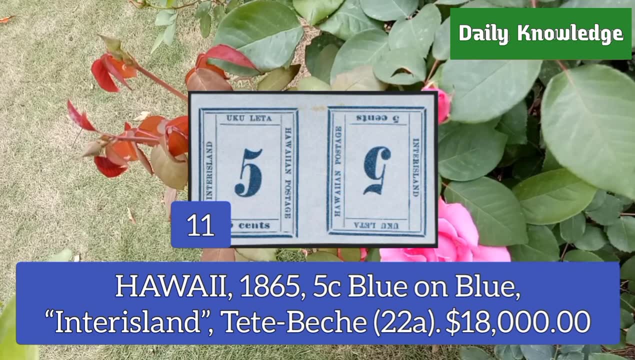 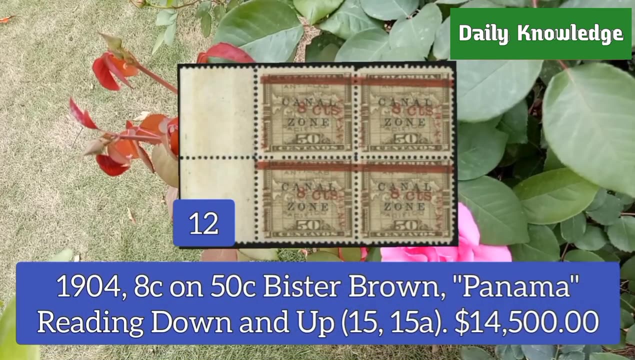 Next is Soldierswear, Stanford, 15 cent pale brown, Scott number WV15.. It is with original gum. Then Hawaii, 1865, 5 cent blue on blue and it is a tete peach pair. 1904, 8 cent on 50 cent. Wester brown, Panama, reading down and up: 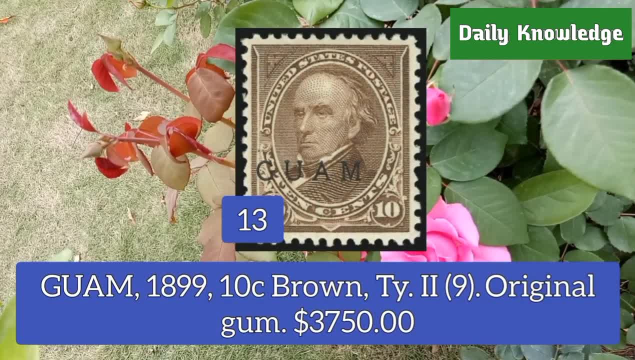 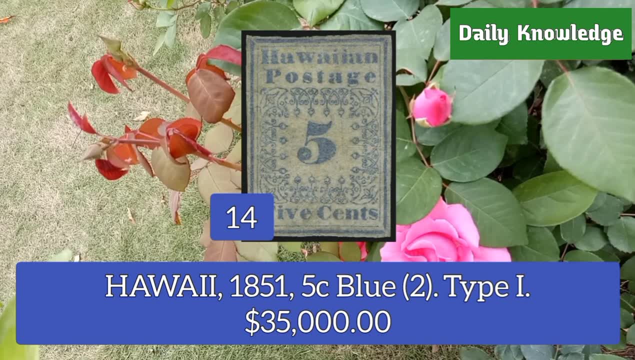 Now Guam 1899, 10 cent brown, type 2, Scott number 9,, it is with original gum. Now Hawaii 1851, 5 cent blue, type 1, and it is Scott number 2.. 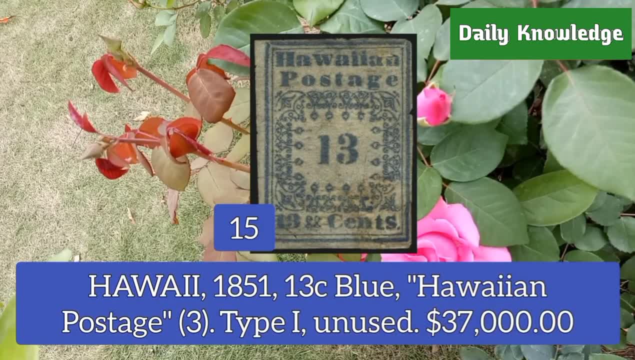 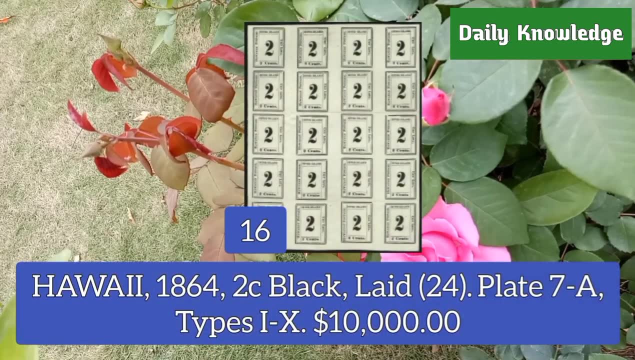 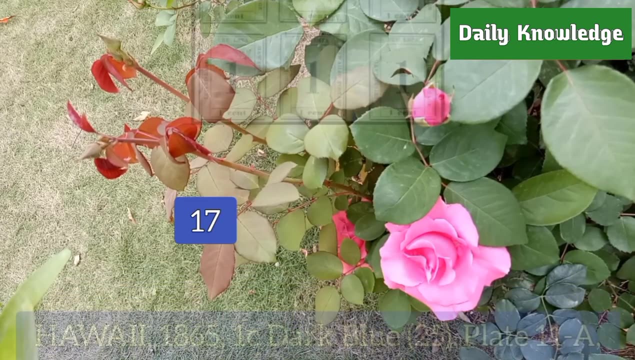 Now, next is Hawaii 1851, 13 cent blue Hawaiian postage and it is Scott number 3, type 1, and it is unused Again. Hawaii 1864, 2 cent black on laid paper, and it is Scott number 24,, plate 7A. 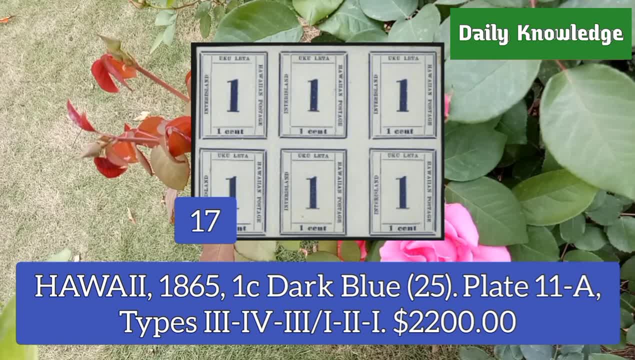 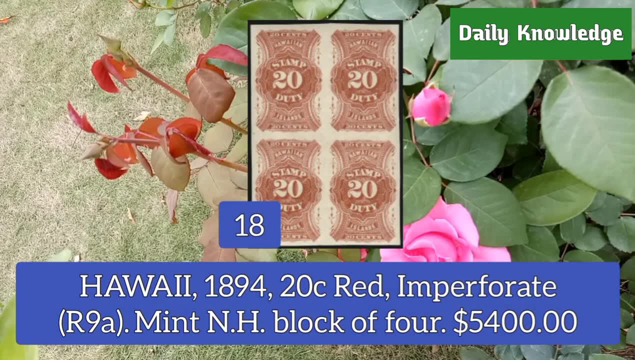 Then Hawaii, 1865, 1 cent dark blue Scott number 25, plate 2A. Next is again from Hawaii, 1894, 20 cent red color in perforate. Next is again from Hawaii, 1895, mint, never hitched, block of 4, Scott number R9A. 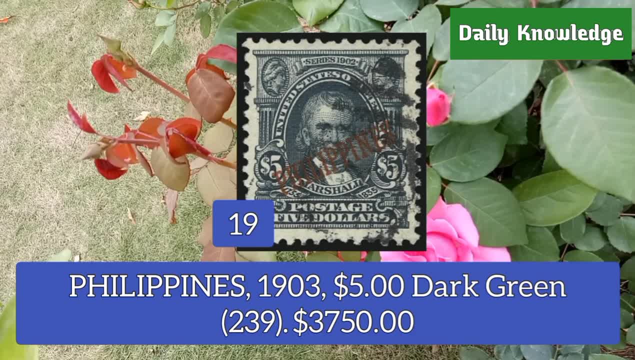 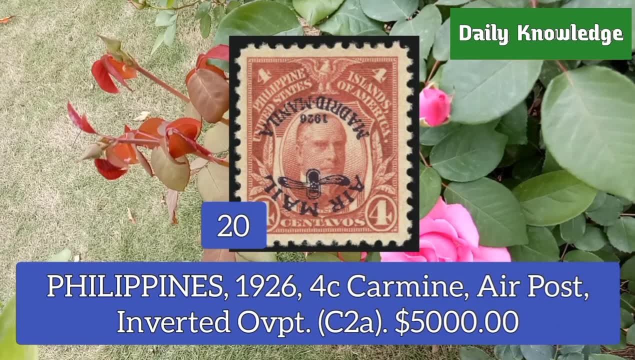 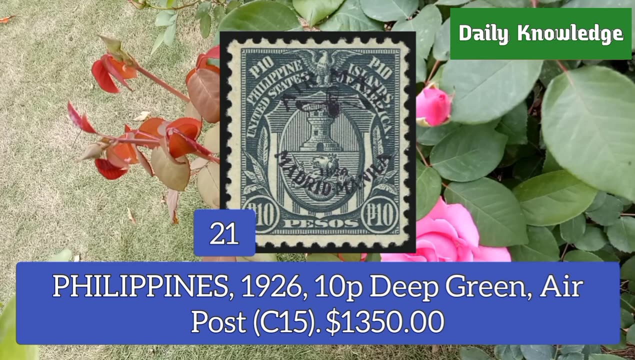 Philippines 1903, 5 dollar, dark green, and it is Scott number 239.. Now it is again Philippines 1926, 4 cent carmine air post, inverted overprint, Scott number C2A. Philippines 1926, 10 P deep green air post, Scott number C15.. 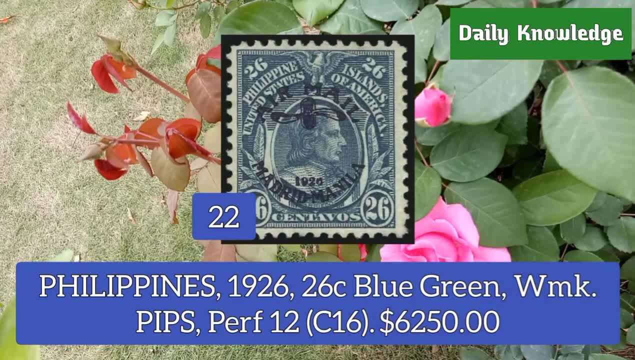 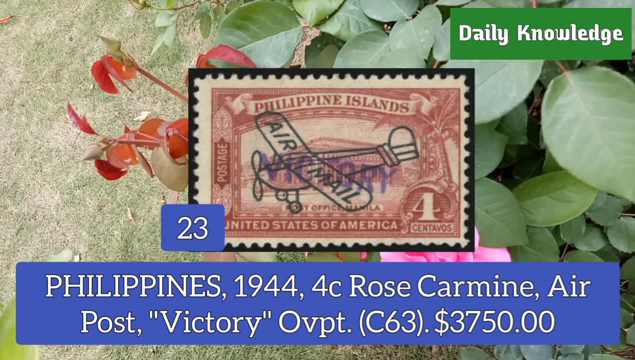 Next is Philippines 1925.. Next is Philippines 1926, 26 cent blue green watermark pips and it is perforation 12. Philippines 1944, 4 cent rose carmine air post victory overprint and Scott number C63. 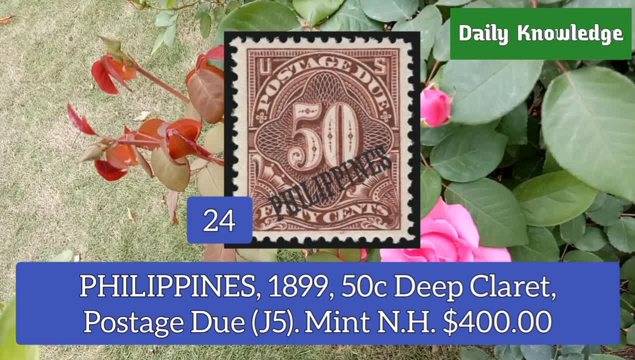 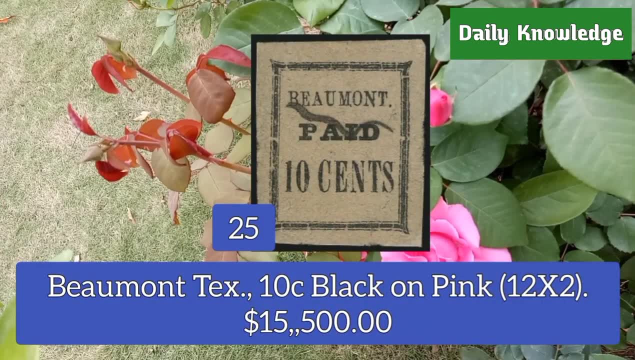 Philippines, 1899, 50 cent deep claret postage due Scott number J5, and it is mint, never hitched. Now. next is Beaumont X, 10 cent, black on pink and Scott number 12X2.. 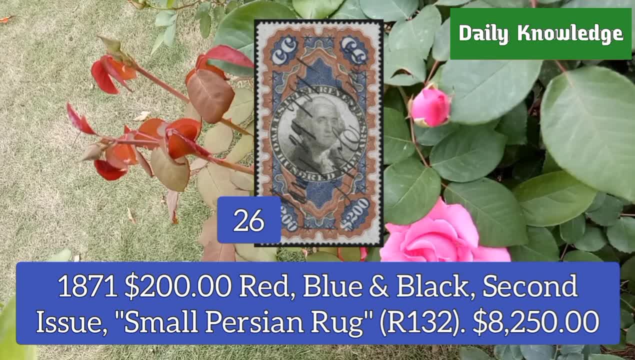 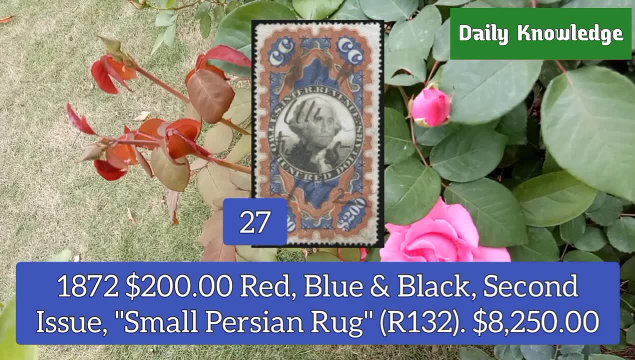 Next is 1871, 200 dollar red, blue and black. second issue, small Persian rug, Scott number R132.. 1872, 200 dollar red, blue and black. second issue, small Persian rug, and it is also Scott number R132.. 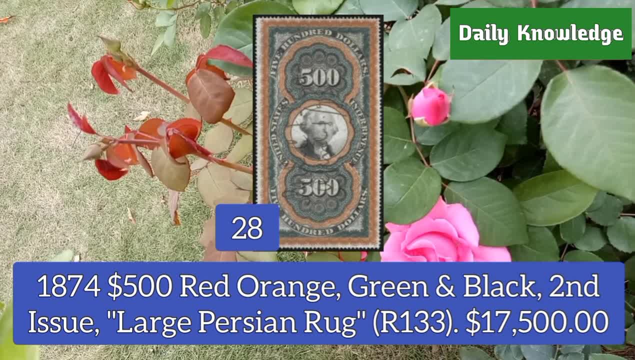 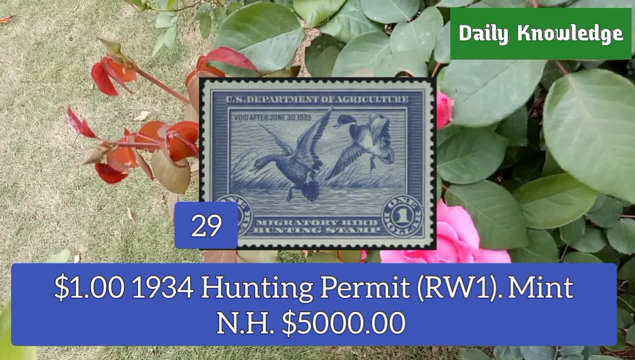 Now 1874, 500 dollar red, orange, green and black. second issue: large Persian rug, Scott number R133.. 1 dollar, 1934, hunting permit, Scott number RW1.. It is mint, never hitched. 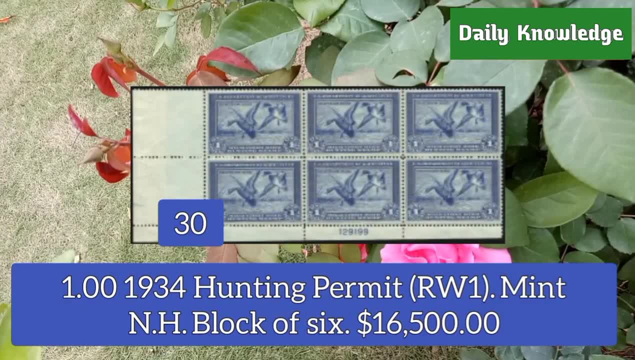 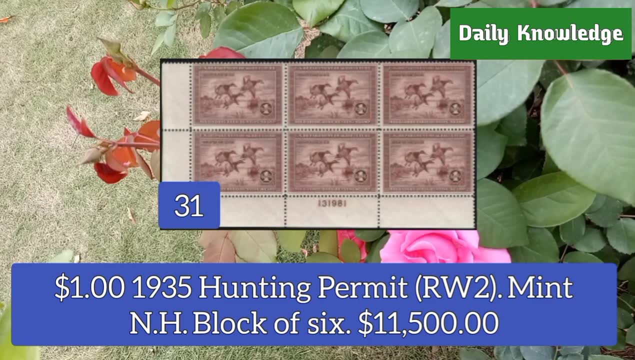 Now: 1 dollar 1934, hunting permit, Scott number RW1.. It is a mint, never hitched block of 6.. 1 dollar 1935, hunting permit, Scott number RW2, mint, never hitched, block of 6.. 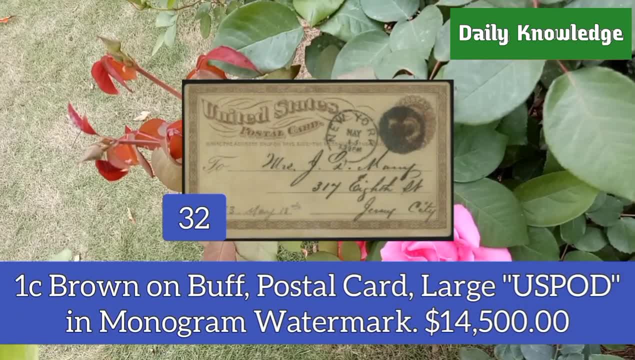 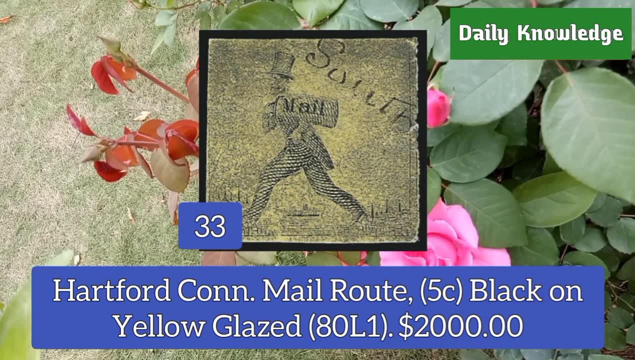 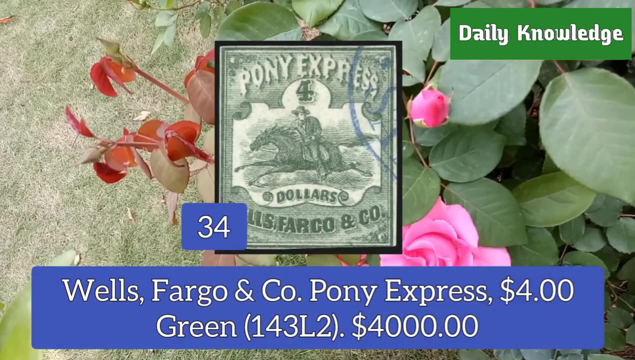 Now 1 cent brown on buff postal card, large USBOD in monogram watermark. Next is Hartford meal route. Black on yellow glazed paper and it is Scott number 80L1.. Wells Fargo & Company, Pony Express. 4 dollar green color and it is 143L2, Scott number. 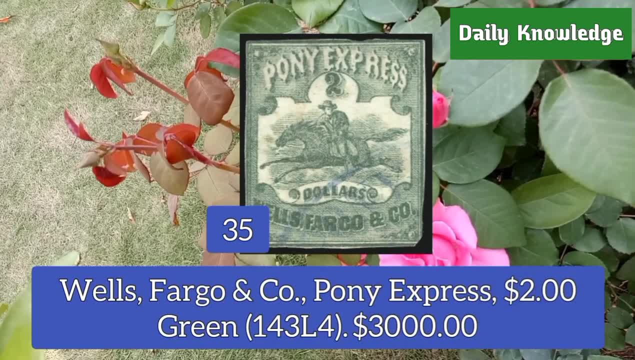 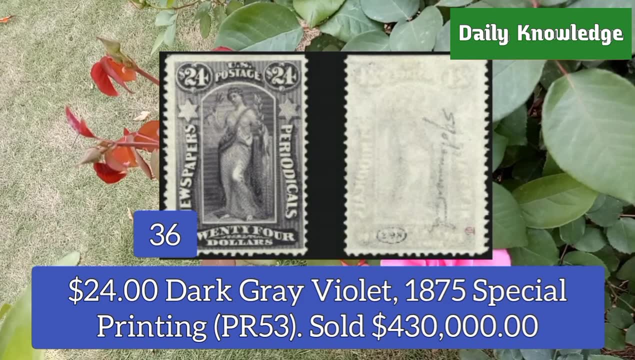 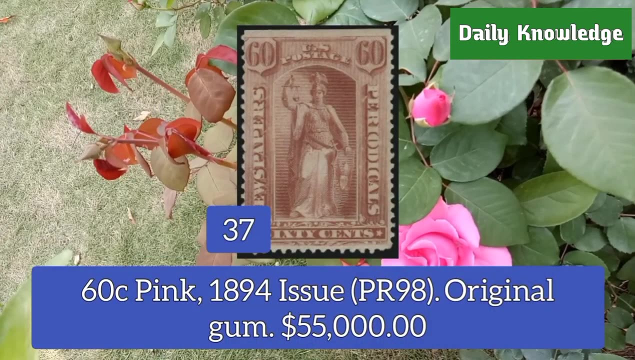 Wells Fargo & Company. Pony Express: 2 dollar green color. 143L4 is the Scott number. 24 dollar dark gray violet, 1875,. special printing PR53 is the Scott number. 60 cent pink, 1894,. issue Scott number PR98, and it is with original gum. 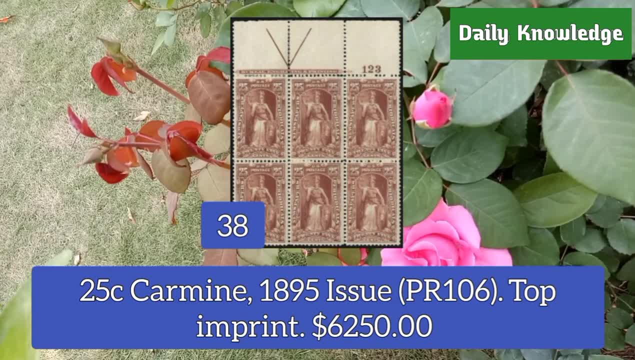 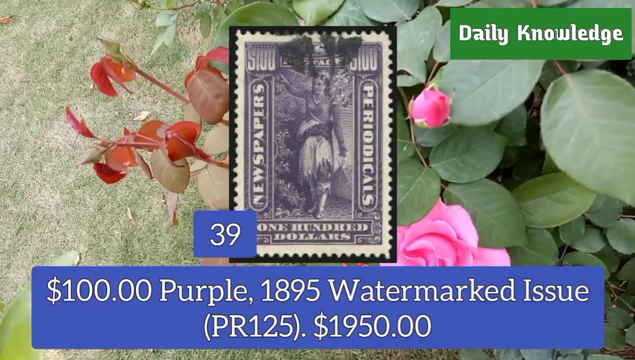 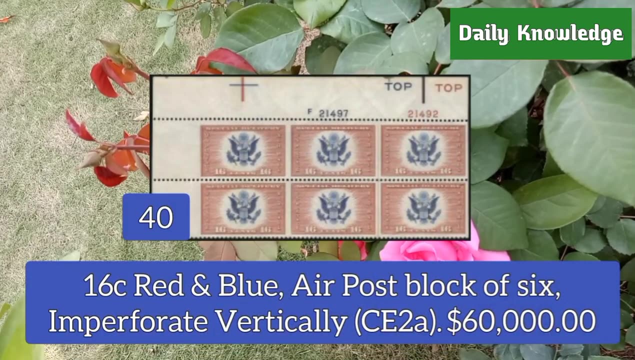 25 cent carmine, 1895, issue, and it is Scott number PR106, and it is top imprint. 100 dollar purple, 1895, watermarked issue, and it is Scott number PR125.. Now 16 cent red and blue air post block of 6, imperforate vertically, Scott number CE2.. 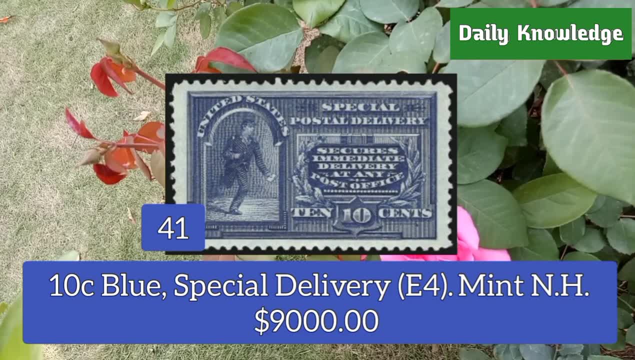 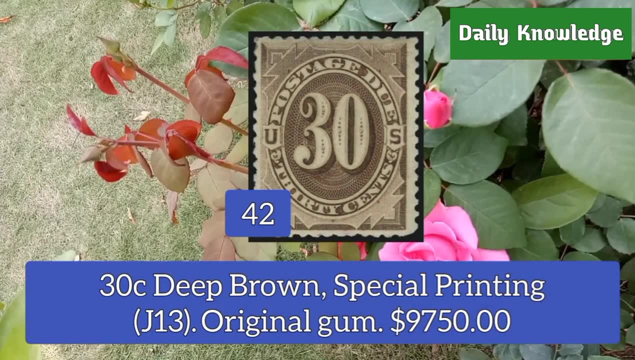 Now next is 10 cent blue color special delivery. E4 is the Scott number and it is mint, never hinged. 30 cent deep brown special printing Scott number J13, and it is with original gum. 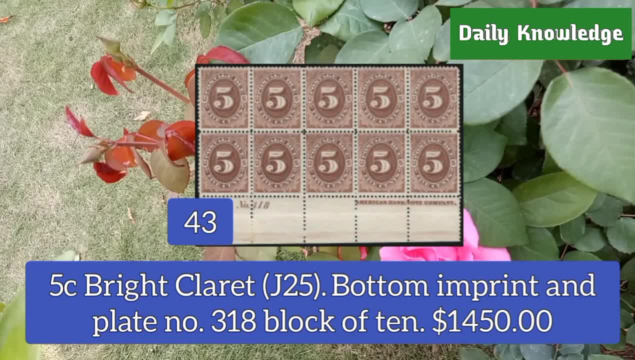 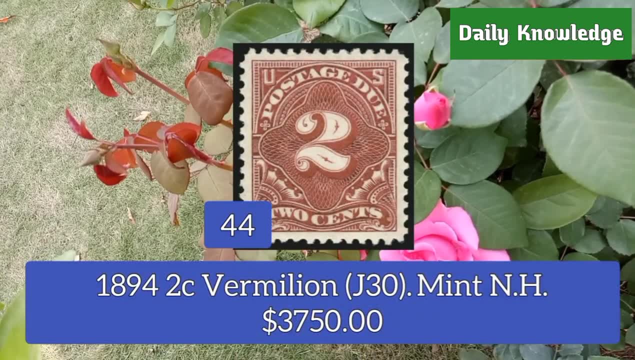 Next is 5 cent bright colored Scott number J25, it is bottom imprint and plate number 318, block of 10.. Now this is 1894,. 2 cent vermilion and it is Scott number. 20 cent red and blue and it is Scott number J13, it is unused mint, never hinged. 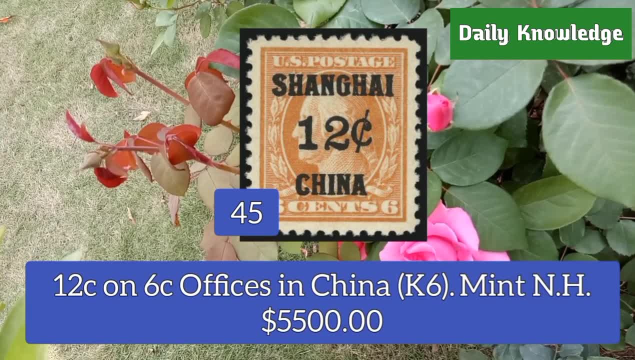 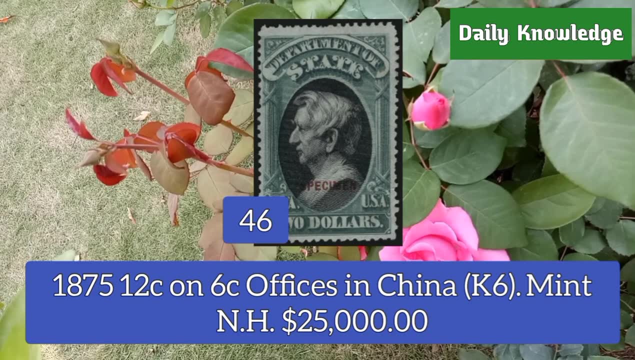 12 cent on 6 cent office in China. it is Scott number K6, and it is mint never hinged. Now, 1875, 12 cent on 6 cent office in China, Scott number K6,, it is mint never hinged. 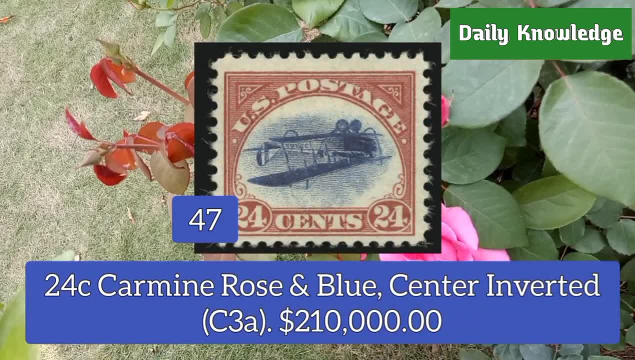 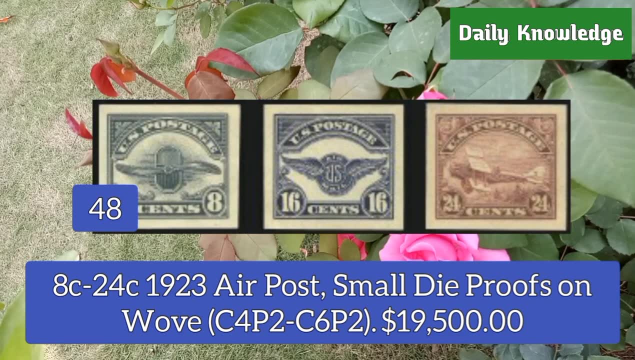 Now next is 24 cent carmine, rose and blue center inverted, and it is Scott number C3A, 8 cent to 24 cent 1995.. 1923, airport stamp- small die proof on wove paper. 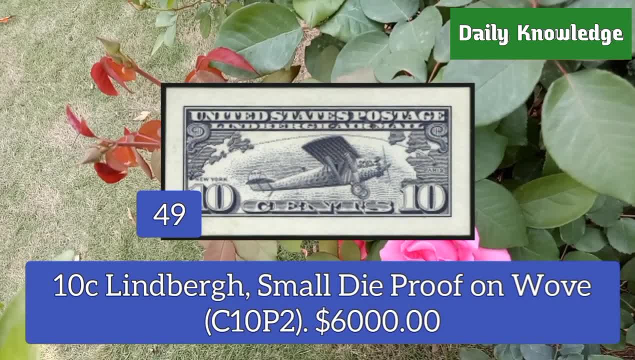 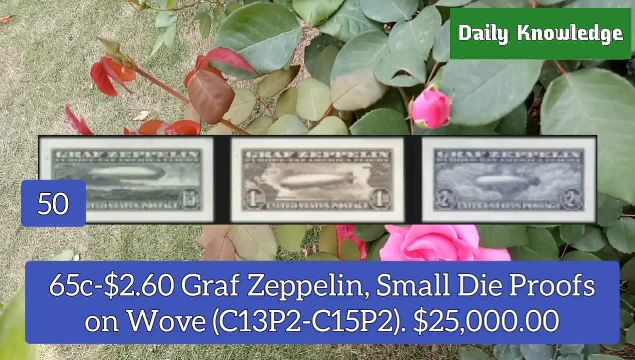 Now, next stamp is 10 cent Lindbergh, small die proof on wove paper, and it is Scott number C10B2.. Now this is 65 cent to 2.60, graph sapling issue: small die proofs on wove paper. 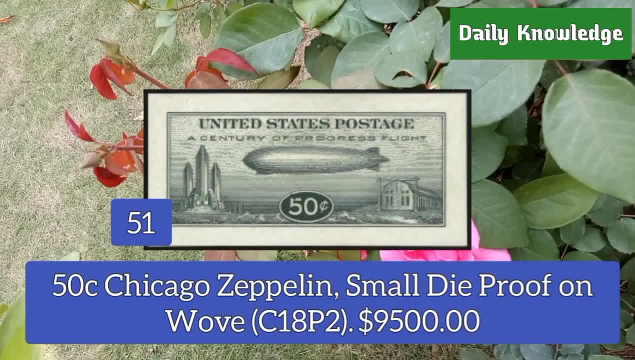 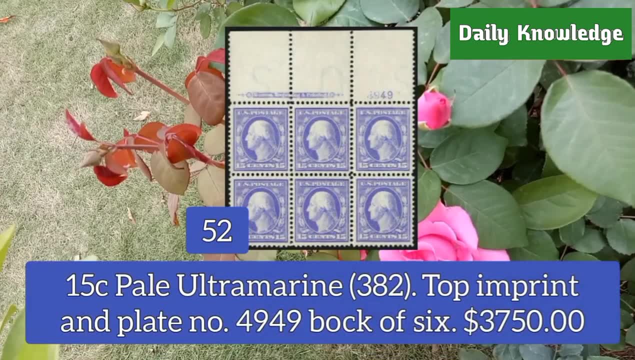 Next stamp is 50 cent Chicago sapling, small die proof on wove paper and Scott number is C18B2.. Now this is 15 cent pale ultramarine, Scott number 382, it is a top imprint- and plate number 4949, block of 6.. 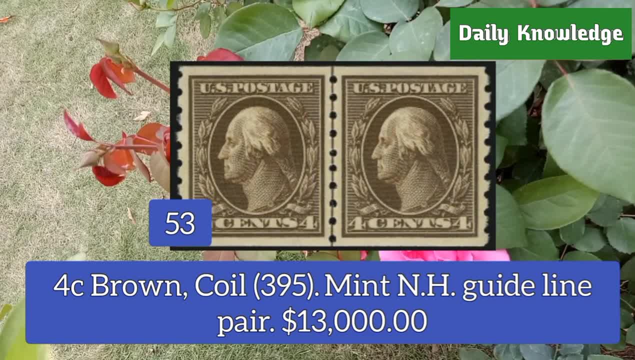 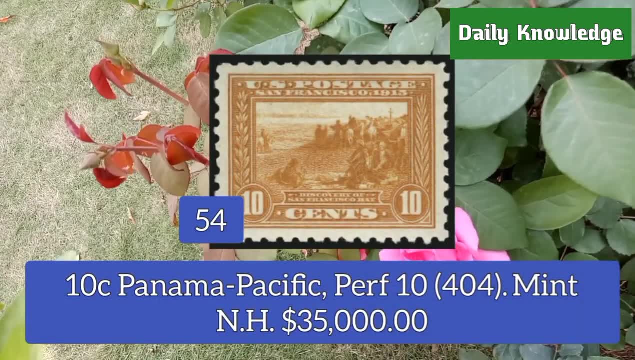 4 cent brown coil stamp 395,. Scott number: it is mint, never hinged. guideline pair. This is 10 cent Panama Pacific perforation 10,. it is Scott number 404, it is also mint, never hinged. 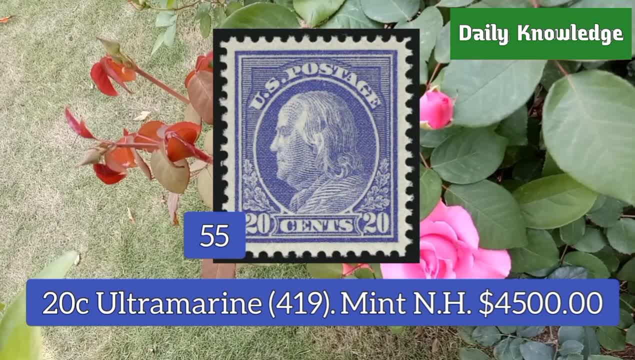 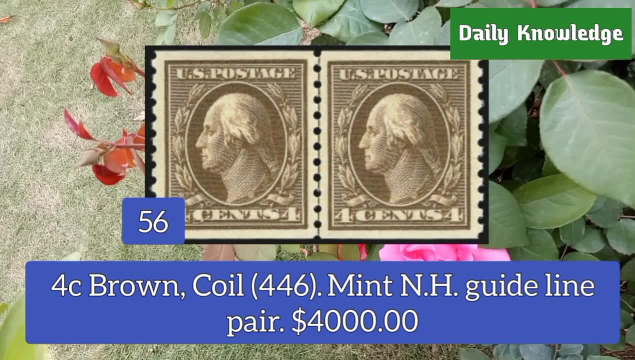 20 cent ultramarine Scott number 419, and it is mint, never hinged. It is unused. Next is 4 cent brown coil stamp Scott number 446,. it is mint, never hinged. guideline pair. 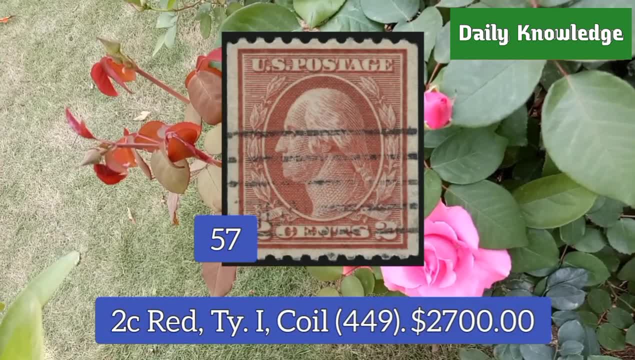 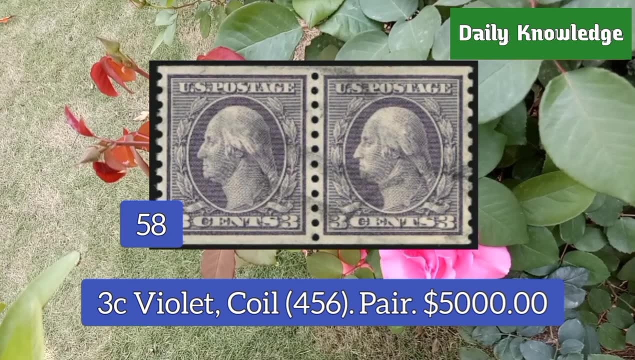 This is 2 cent red color type 1, coil stamp and it is Scott number 449,. it is a used example. Now, 3 cent violet coil stamp, Scott number 456, and it is a pair. 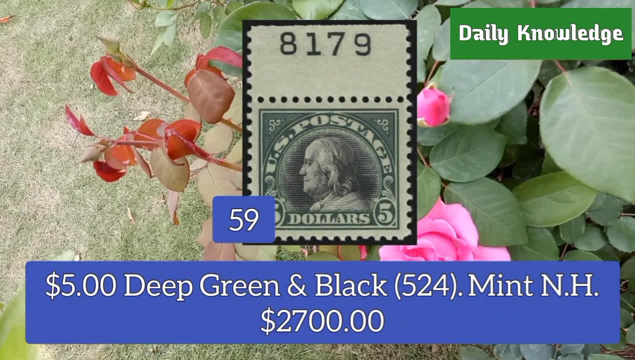 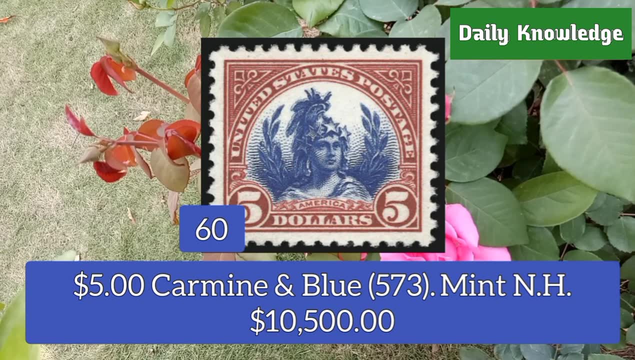 Next is 5 dollar deep green and black- Scott number 456.. It is Scott number 524, and it is mint never hinged. Now next is 5 dollar Carmine and blue Scott number 573, and it is mint never hinged. 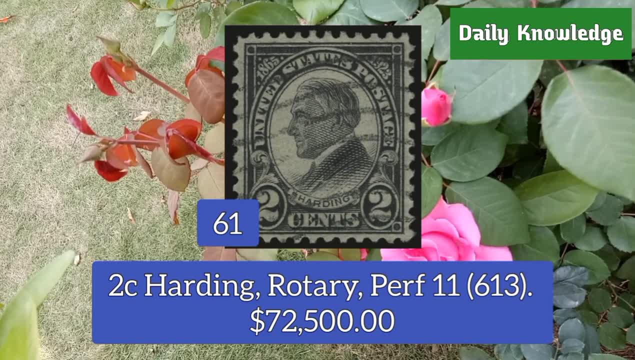 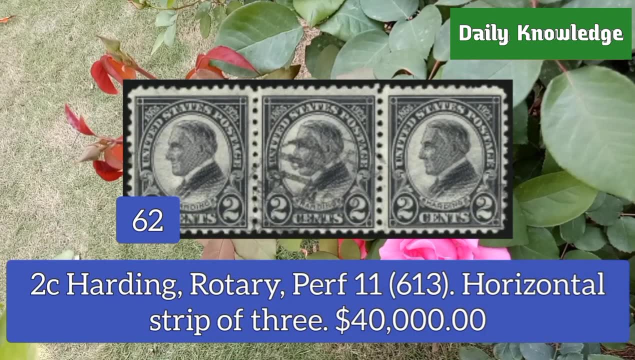 It is unused. 2 cent harding rotary perforation 11, Scott number 613.. Next is 2 cent harding rotary perforation 11, Scott number 613.. It is a horizontal strip of 3.. 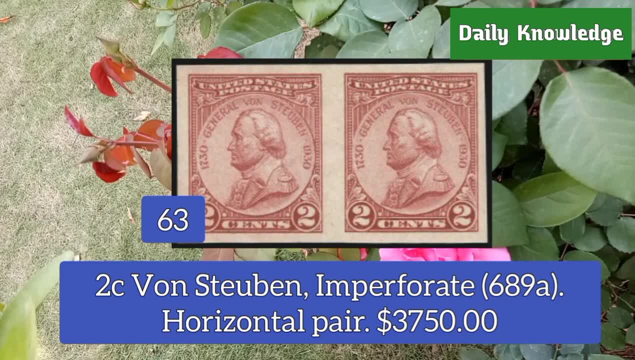 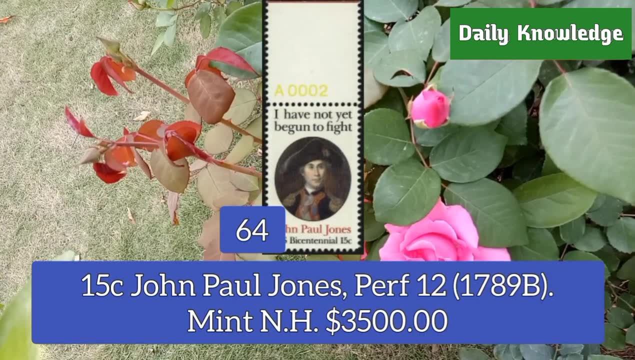 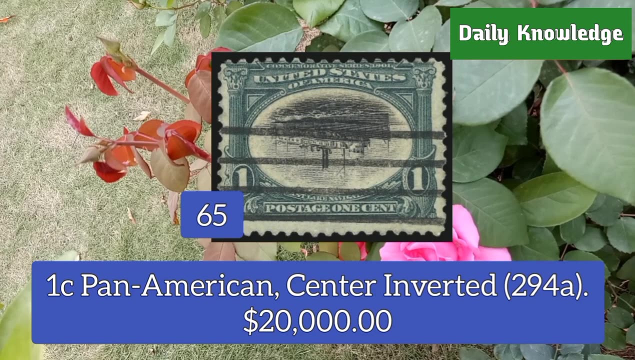 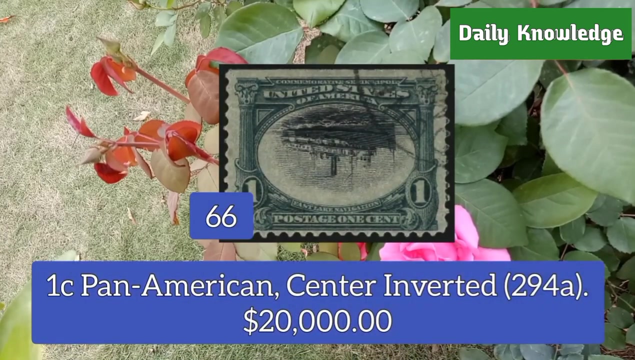 now two cent one steuben in perforate. score number 689a and it is a horizontal pair. now this is 15 cent. john paul jones, perforation, 12.. score number 1789b: now this is one cent pan american center inverted. it is a used example and it is caught. number 294a, one cent pan american center inverted. 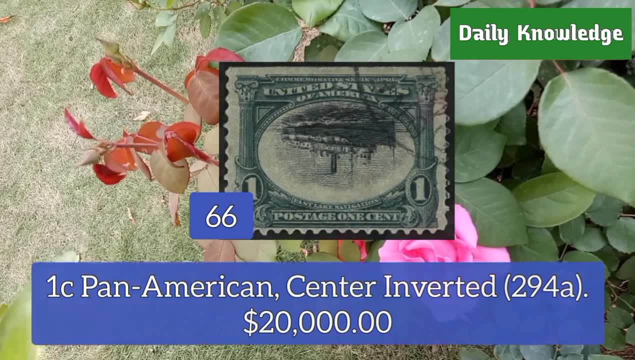 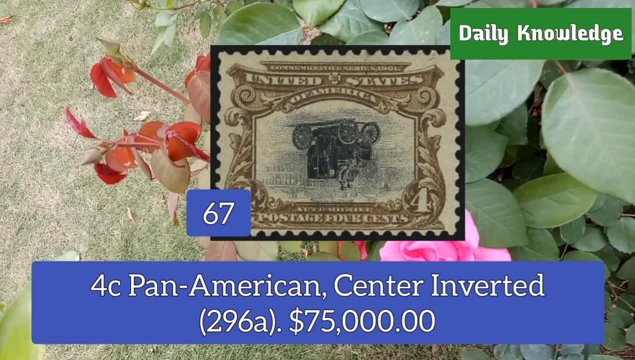 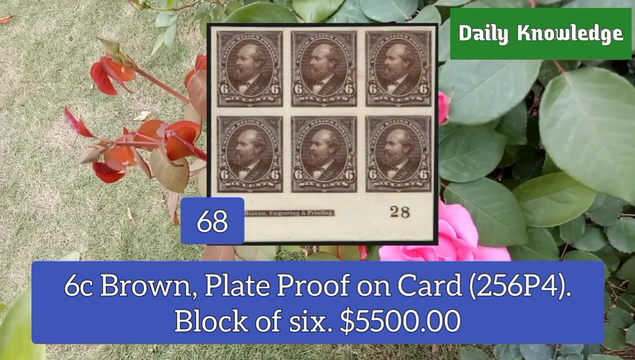 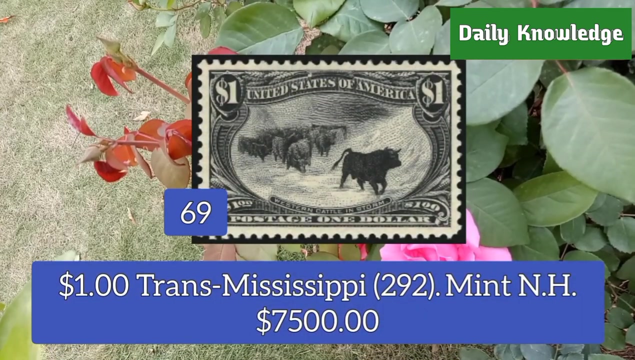 scored number 294a. it is also used now. next is four cent pan-american center inverted and squad number is 296a. next is six and brown plate proof on card block of six and the score number is 256b4. now this is one dollar trans mississippi issue and it is got number 292. 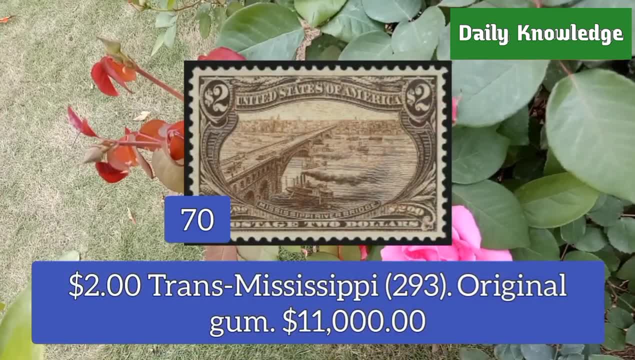 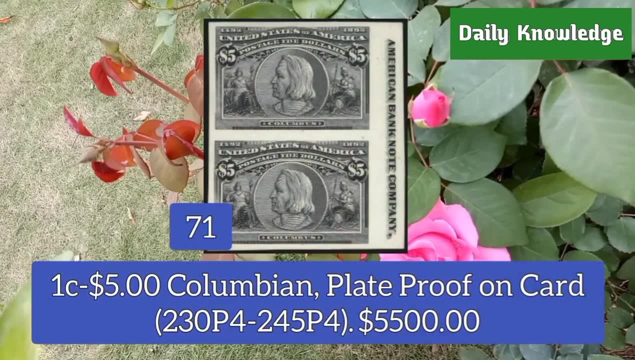 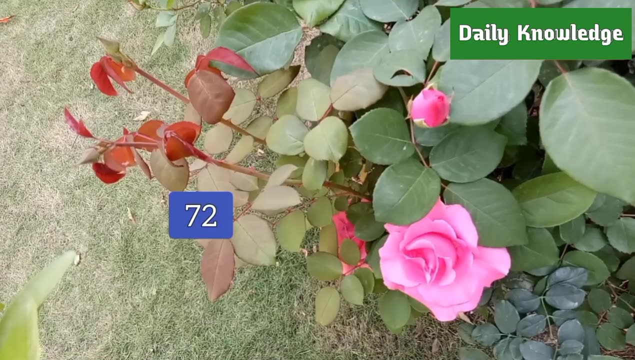 it is unused mint never hunched to $2 transmissive PSU Scott number 293 and it is also unused with original gum. this is one cent to five dollar. columbian plate proof on card Scott number 230p4 to 245p4- four cent. 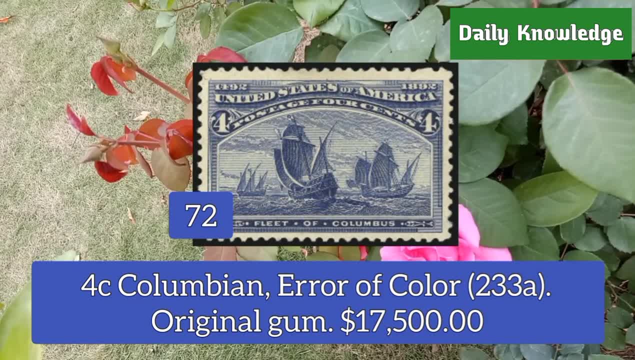 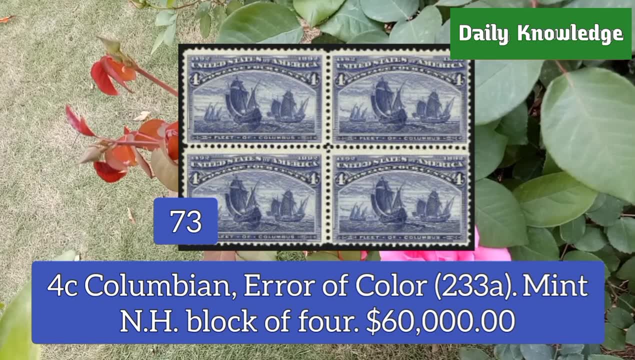 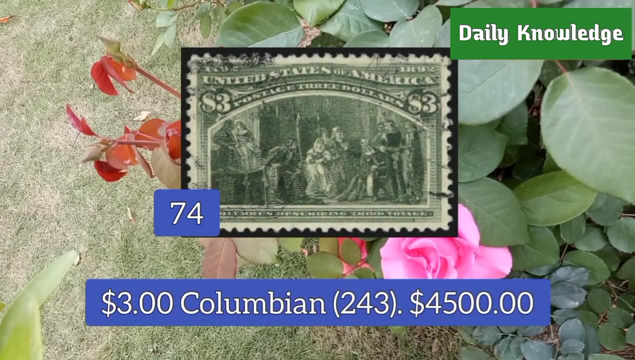 columbian error of color Scott number 233a and it has original gum now. next is four cent columbian error of color Scott, number 233a and it is a mint averaged block of four three dollar. columbian Scott number 243, estimated value: four thousand five hundred dollars now. 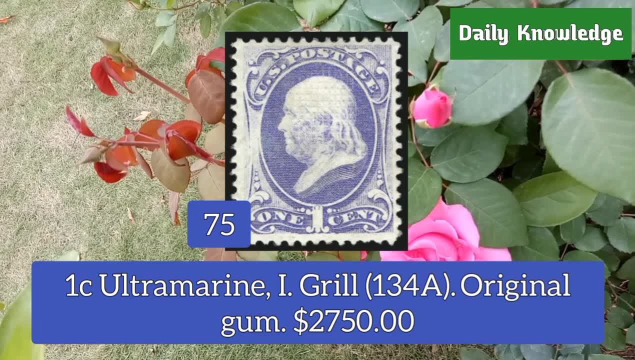 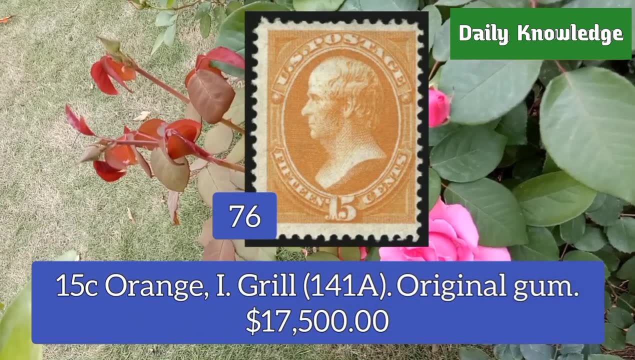 one cent ultramarine eye grill 134a is the Scott number and it is unused with original gum. 15 cent orange eye grill, Scott number 141a and it has original gum. you can also buy this product from the link in the description box below this video and. 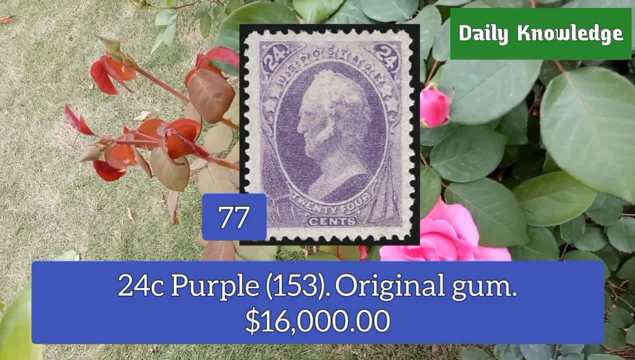 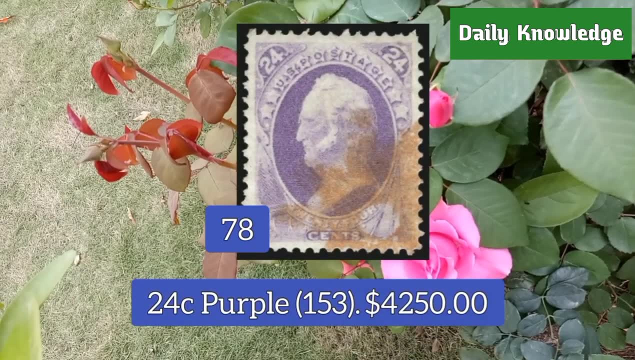 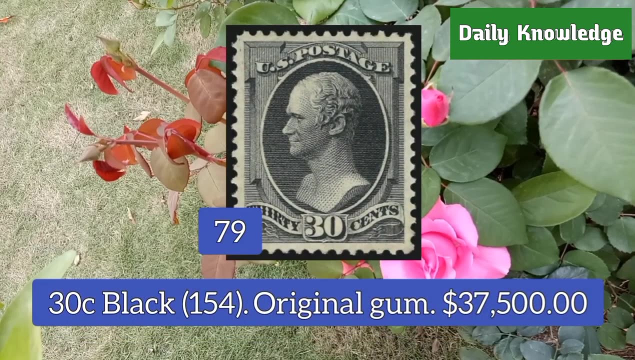 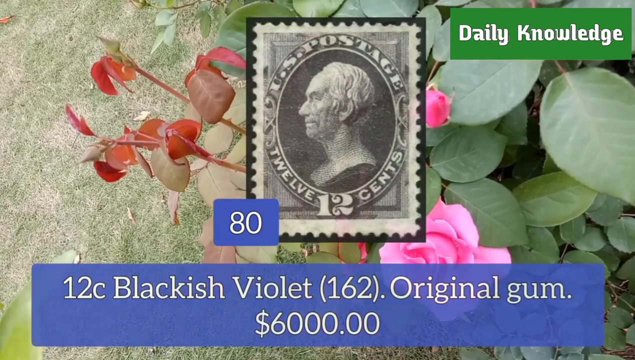 now. next us stamp is 24 cent purple color and it is Scott number 153. it is also unused with original gum. this is 24 cent purple, Scott number 153. now it is a used example. then 30 cent black color, Scott number 154, and it has original gum. now next is 12 cent blackish violet, Scott number 162, and it has. 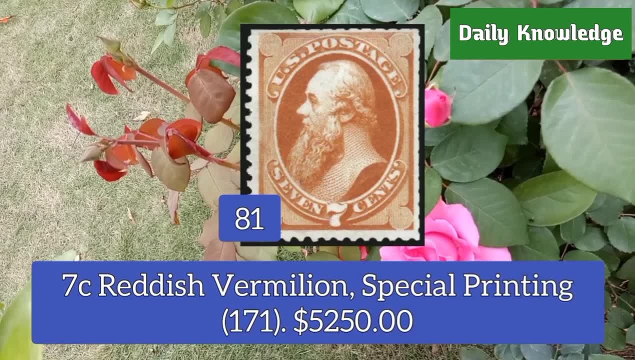 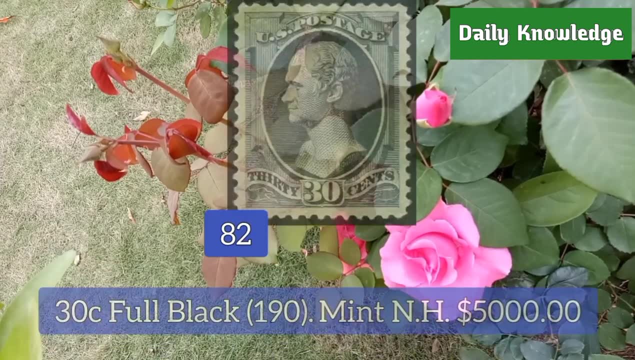 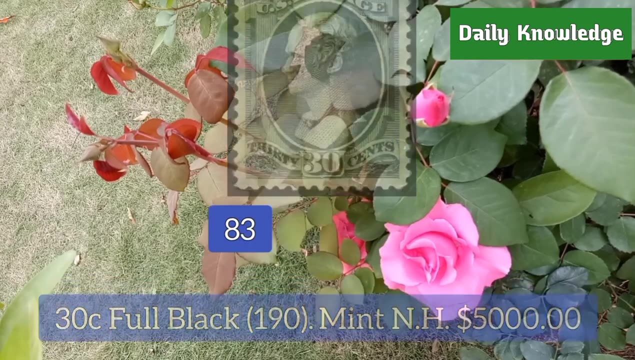 original gum. now now next is 12 cent orange color and it is a unused example. seven cent reddish vermilion special printing, Scott number 171. it is also unused. 30 cent full black Scott number 190, mint, never aged, unused example. now next stamp is five cent indigo Scott, number 216. it is a unused 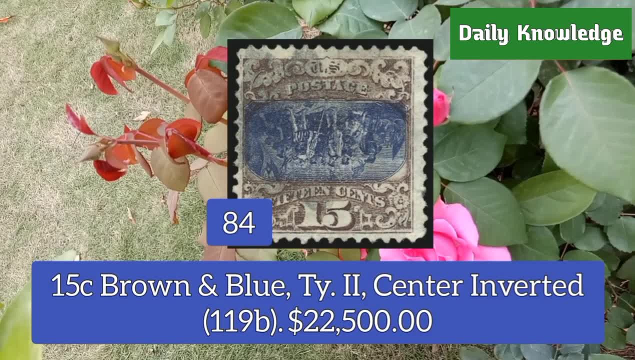 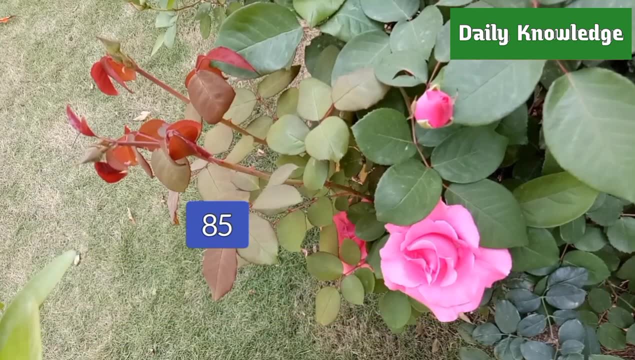 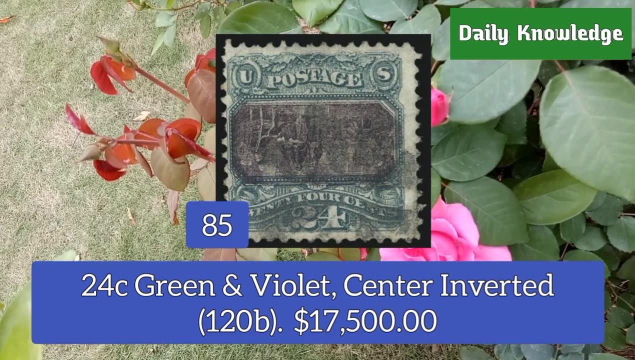 example, and it is mint, never hinged. next is 15 cent brown and blue type two, and it has original center inverted, and it is caught. number 119b: 24 cent green and violet center inverted, and it is caught. number 120b. next is 30 cent ultramarine and carmine flex inverted. 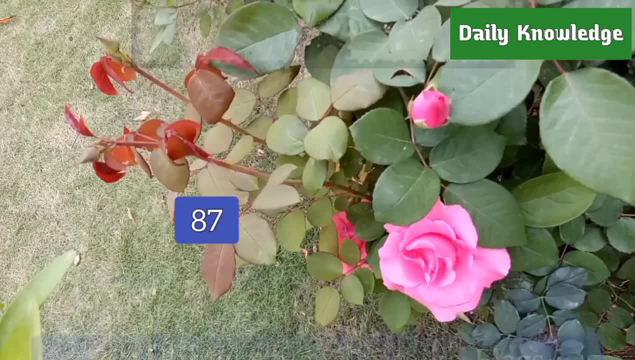 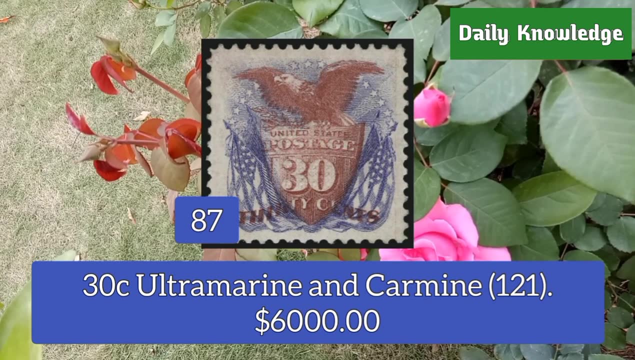 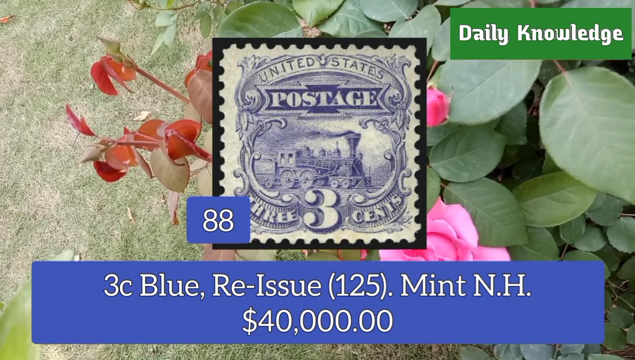 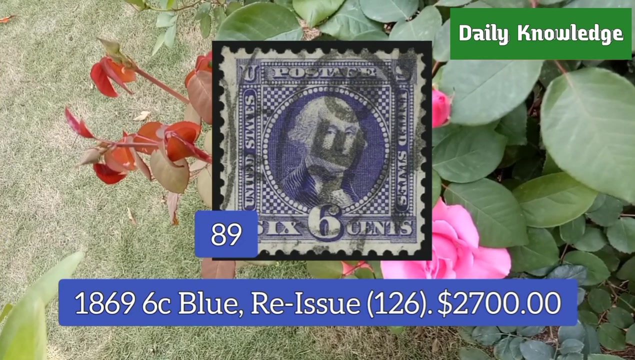 scott number 121b and it is unused. 30 cent ultramarine and carmine scott- number 121, estimated value: 6 000 us dollar. 3 cent blue reissue: scott number 125 and this mint never hinged. now next is 1869, six cent blue color reissue and it is caught. number 126. 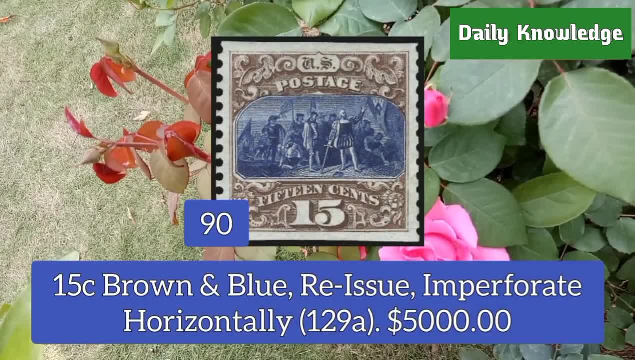 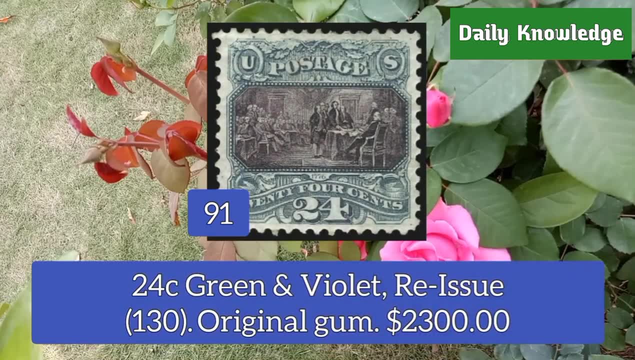 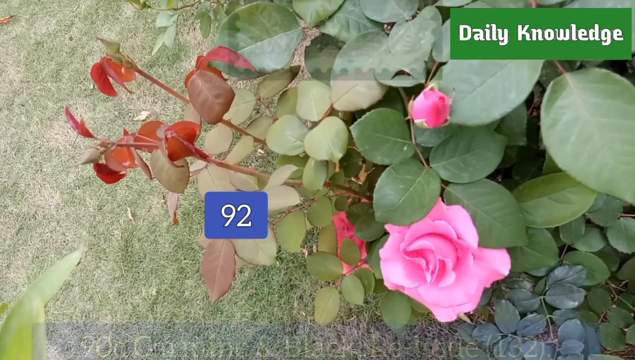 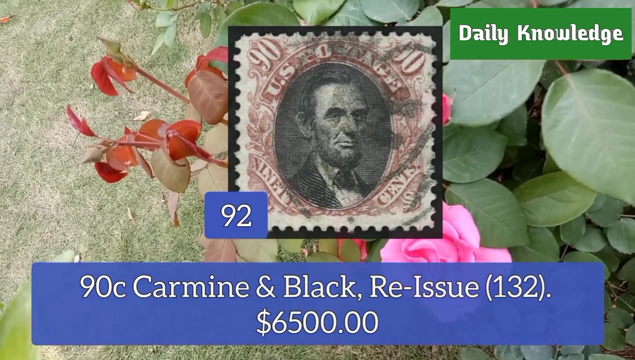 now 15 cent brown and blue reissue, imperforate horizontally- scott number 129a. 24 cent green and violet reissue- scott number 130, and it has original gum now. next is 90 cent carmine and black reissue- abraham lincoln stem and it is caught- number 132. it is a used example. 3 cent green and